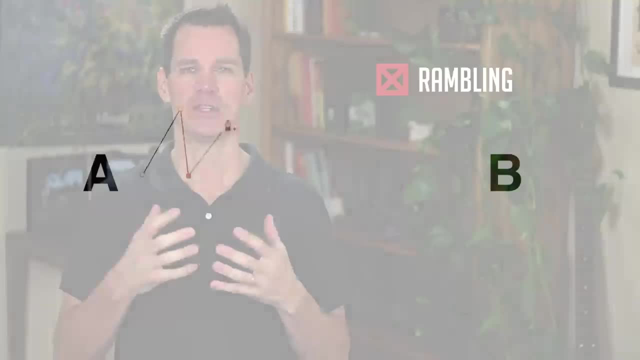 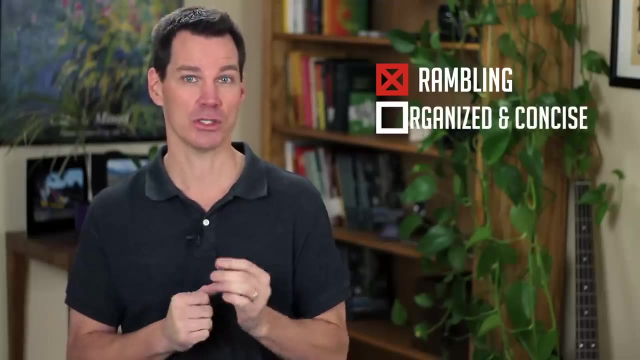 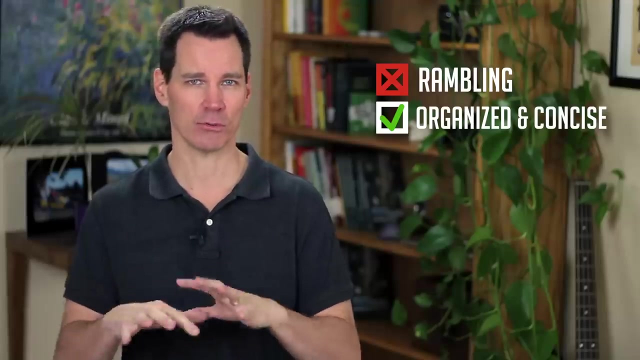 and get long-winded. Anytime a speaker is disorganized and weaves all around, it's very hard to follow what he or she is talking about, And instead what you want to do is give a nice, organized and concise message. That means you have to take the time beforehand when you're preparing. 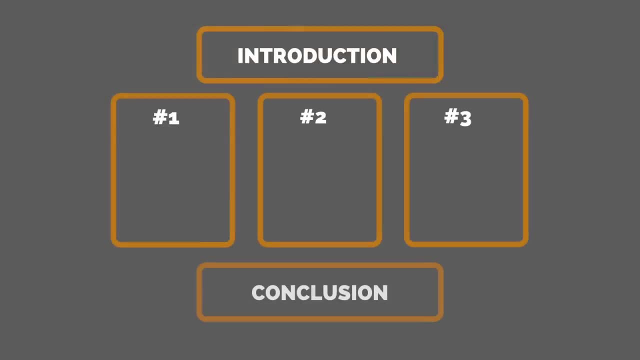 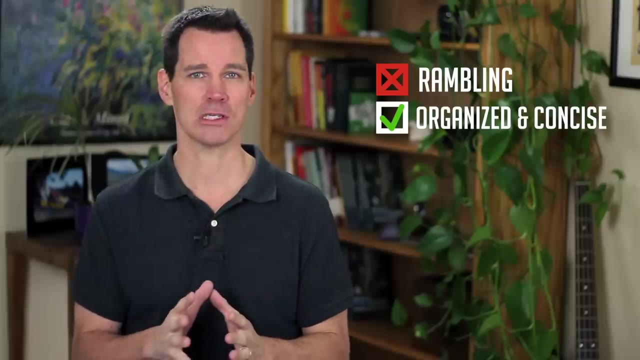 to create a nice introduction body and conclusion, Make sure you have clear main points and there's a transition statement between each main point. Your audience is really going to have an orderly presentation of your ideas and it's much more likely that they'll remember what. 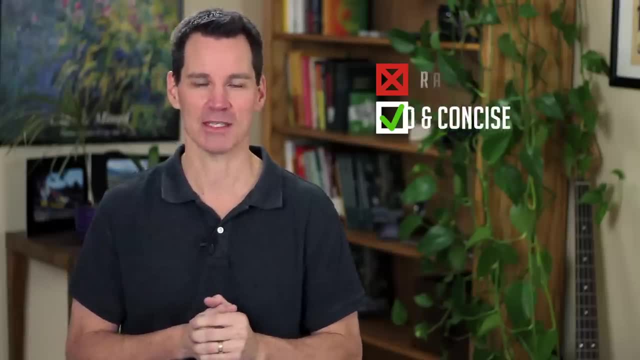 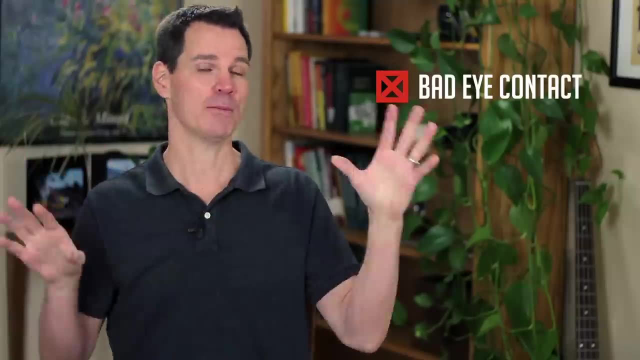 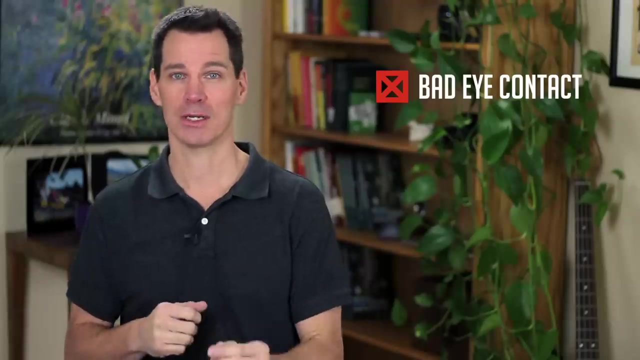 you said- And really that's the whole point of speaking to them in the first place- The next don't is: don't look with your eyes in the wrong places. You want to not look over people's heads or not look at the floor and not stare at the ceiling or scan around like that. What you want. 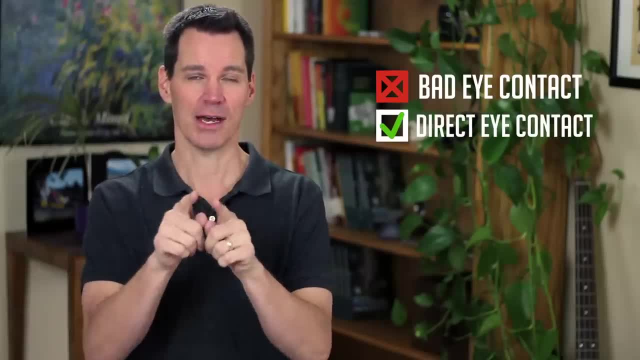 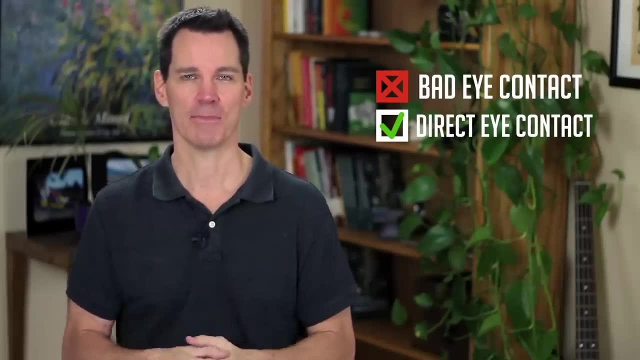 to do is look directly into a person's eye long enough to finish a thought, and then move on and look at the other person's eyes, And that's what we're going to talk about today. So let's get started. Look directly into the next person's eyes long enough to finish a thought. One public speaking. 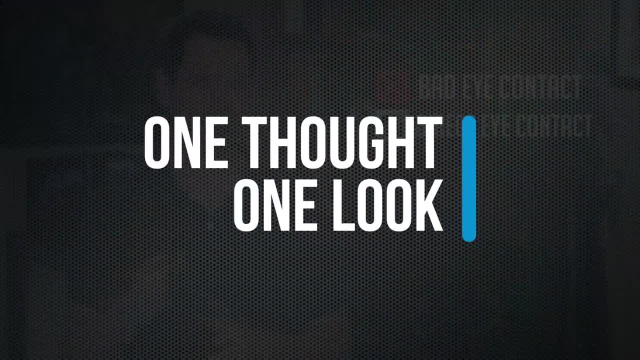 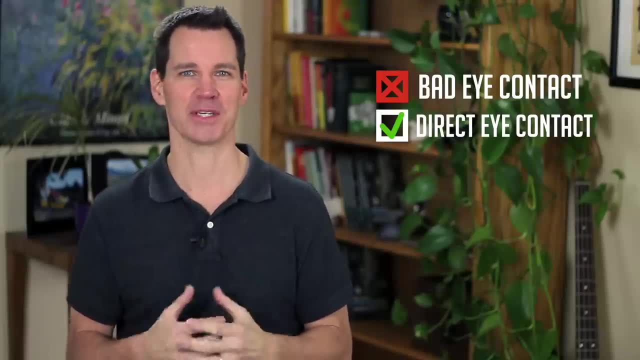 teacher told me one thought: one look, In other words, about a sentence or a half a sentence, and then move on to the next person. Now this is very difficult to do if you're not used to it. It can feel very awkward looking right into someone's eyes, but you have to gear up for this because 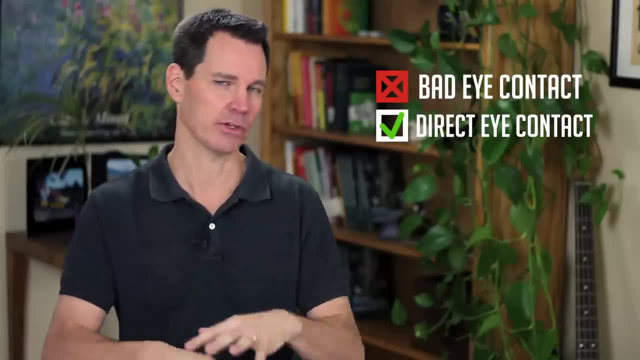 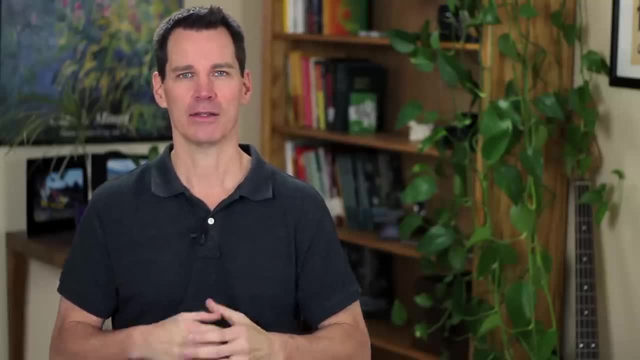 that's what audiences want. We want people to connect with us. If you're not looking into our eyes and making us feel like we're part of this, then you're not going to have much of an impact. The next thing you want to do is: don't- rather, this is a don't- don't- clutter up all your 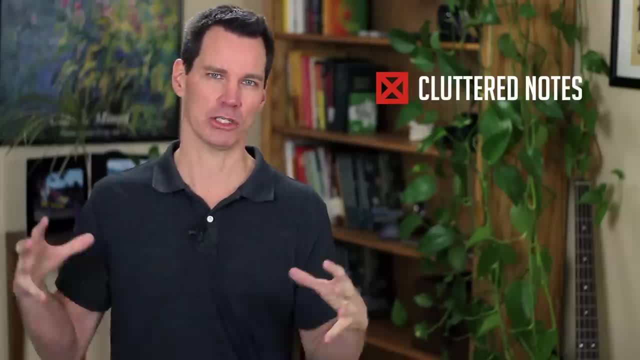 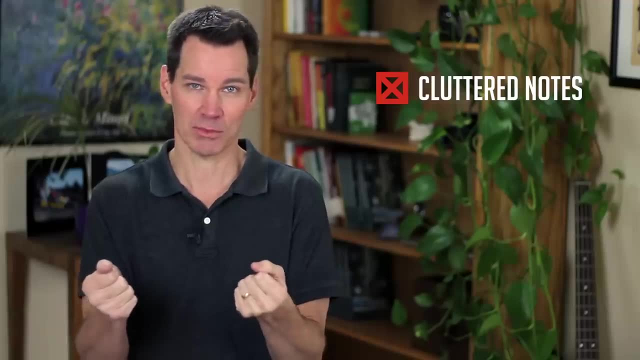 notes with too many details. A lot of times we're tempted to jam our notes or our PowerPoints with everything we want to say, but the result is, when we're nervous in the moment, we end up just locked into our notes and looking down the whole time and reading and sounding really stiff, really. 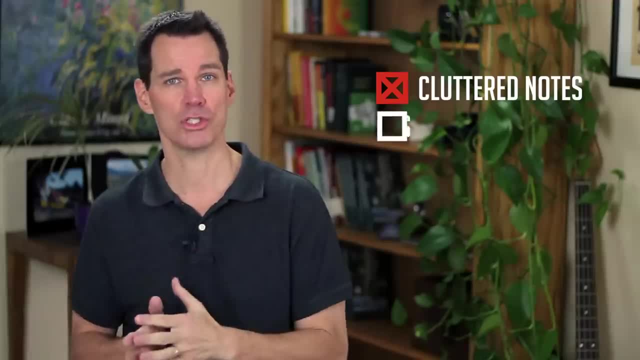 wooden and you're not going to again connect with people. So what you want to do instead is pare down your notes and look at the whole time and reading and sounding really stiff, really wooden, and you're not going to again connect with people. So what you want to do instead is pare down your 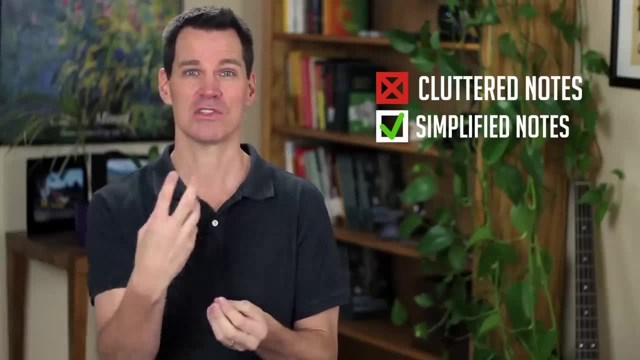 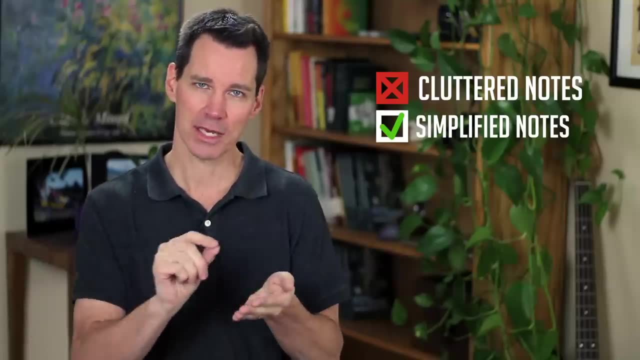 notes so that you can just have a conversational style with your audience. And again, as you're practicing, you have to whittle down those notes so that all you have is like talking points, like a little grocery list of items that you're going to talk about, and it almost forces you, or at 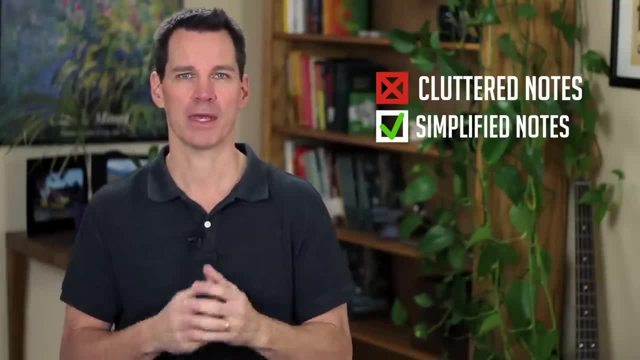 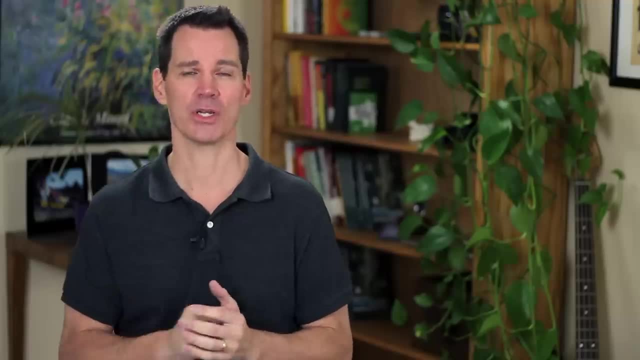 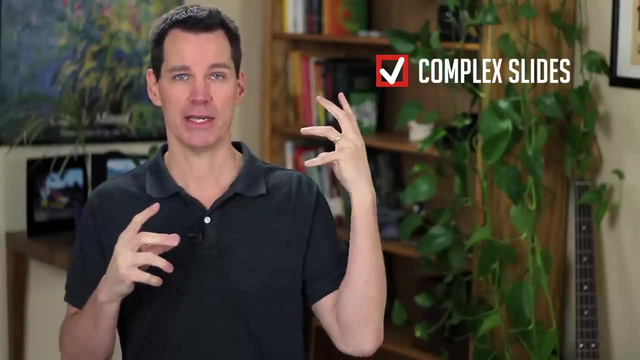 least frees you to connect with people, to look up and to have a nice normal conversation with them and your natural personality. The next don't is you don't want to load up your slides with all complicated animations and text, and one of the reasons is you don't want to stare at it and read from it. The other reason is: 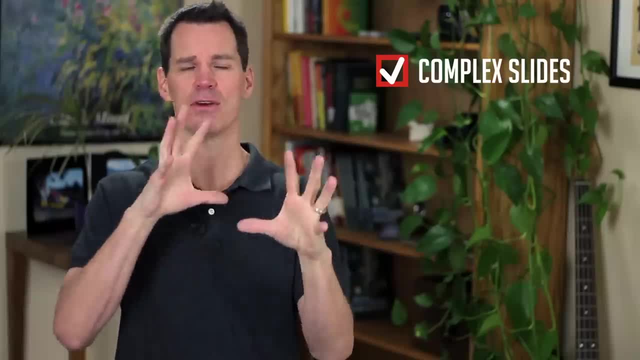 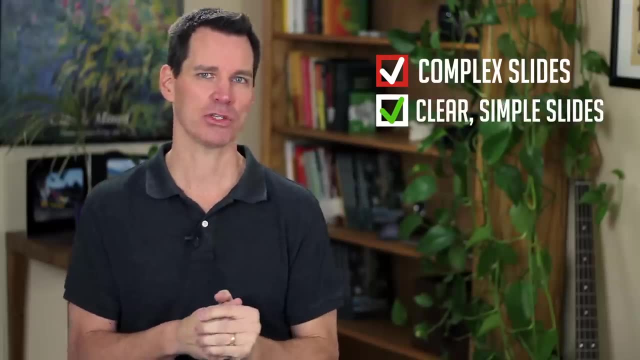 The next don't is. you don't want to stare at it and read from it. The other reason is that it's very hard to follow what's going on if your slides are jam-packed with detail. What you want to do instead is make sure your slides are nice and clear, and 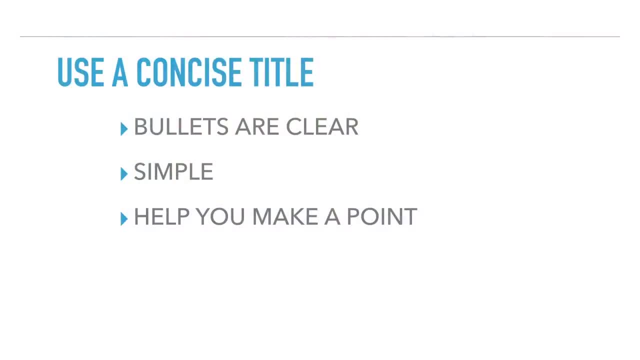 simple and help you make whatever point you're making in that particular moment. A rule of thumb that I like to use is, if you're spending more than about two or three minutes on each PowerPoint slide, I'd peut usering si step si passer seı article um ten souvitory pas de hoje si hair quelque peu więcej than deux ou trois minutes. 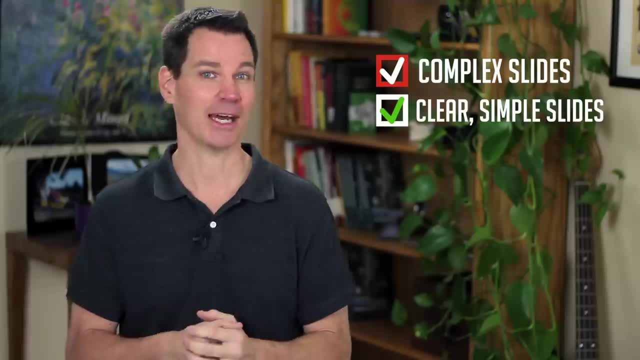 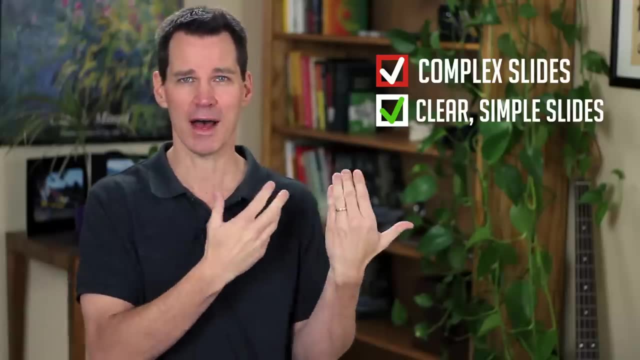 129: 00amy walaikour philosopher que algo pode se uderst避wys slide, then you're probably wasting your time And I don't recommend using more than a couple of slides per presentation. anyway, if you're a beginner- because people tend to over rely on the slides and 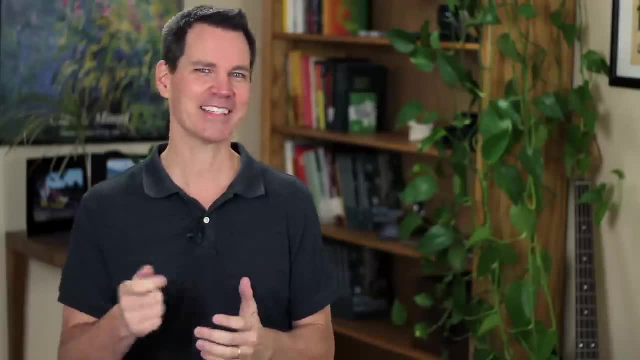 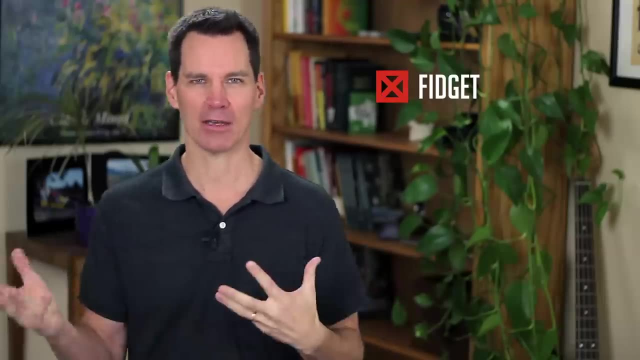 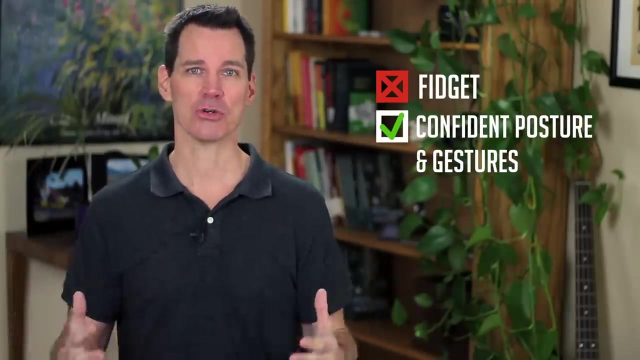 load up each single slide with way too much. The next don't is: don't fidget. Don't fidget with your hands, Don't fidget with your feet, Don't pace back and forth aimlessly because you're nervous. What you want to do instead is have nice confident posture where you stand in one place for a little. 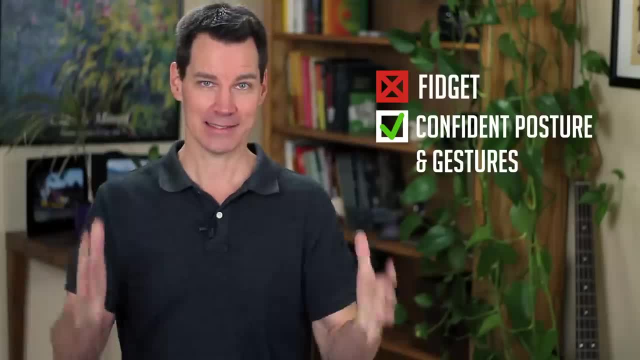 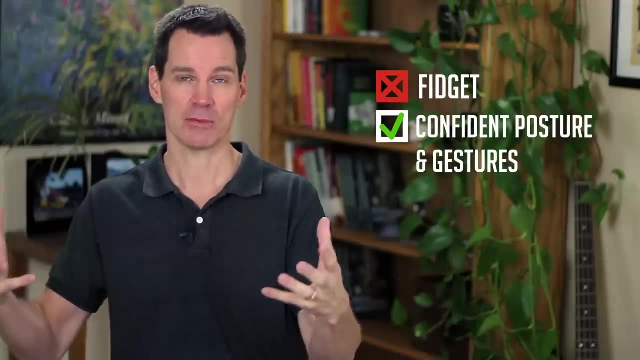 while. And then, if you want to move with a purpose, move, Stand another place for a while and then share another part of your message. Move for the purpose, Stand still. Share some of your message. Don't just pace, Have nice, confident posture. Same thing with your hands. You want to use gestures. 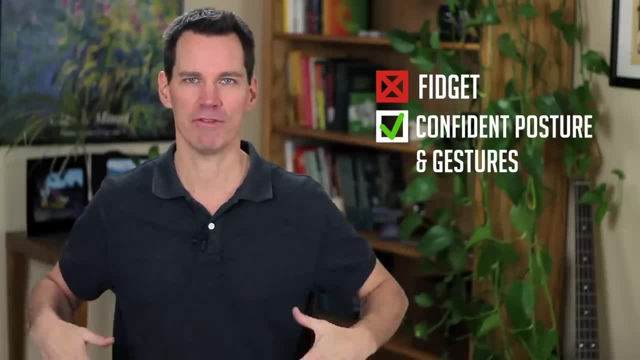 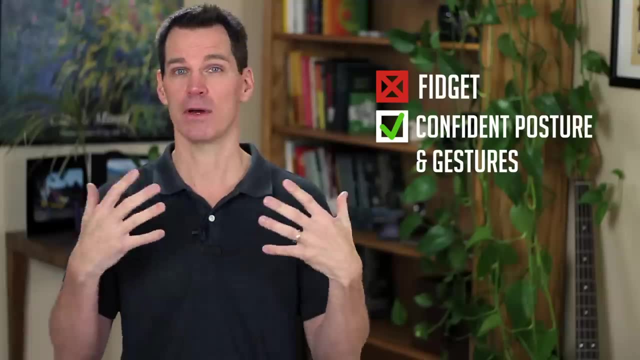 and emphasize your ideas with your hands. You don't want to fidget and put them in your pockets or play with a pen or do anything Anything else weird or distracting like that. That's a big part of how you come across non-verbally.